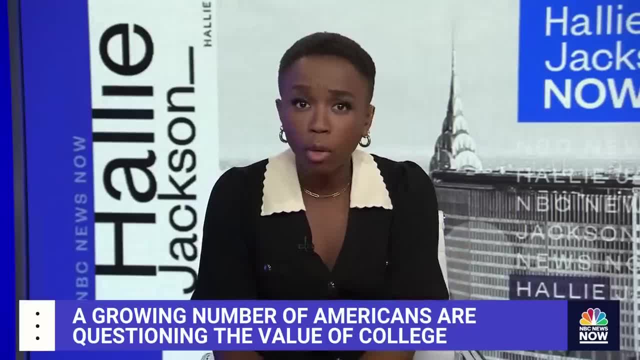 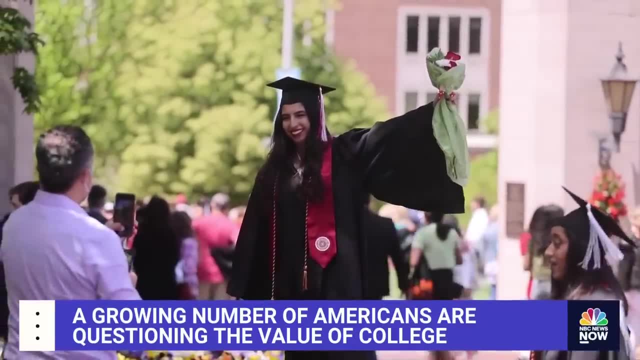 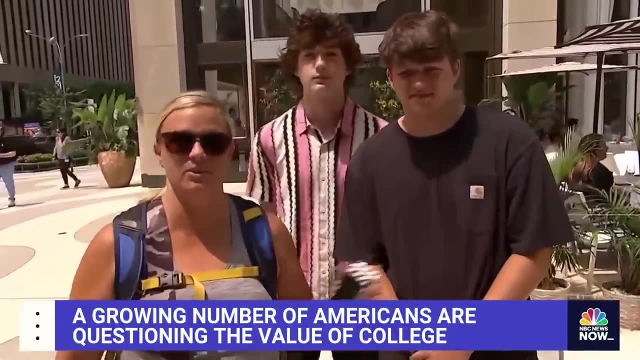 putting college off, dropping out or not going at all. Stephen Romo has more: Getting a college education can be one of the most important financial decisions you'll make in your lifetime. The cost of student college is absolutely insane. He'll be a senior next year and then we'll have to be dealing with that, And we've been looking. 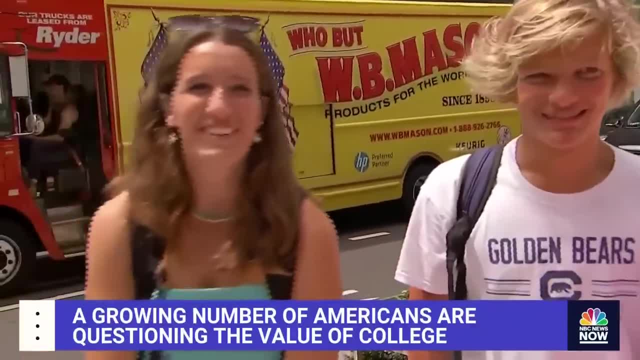 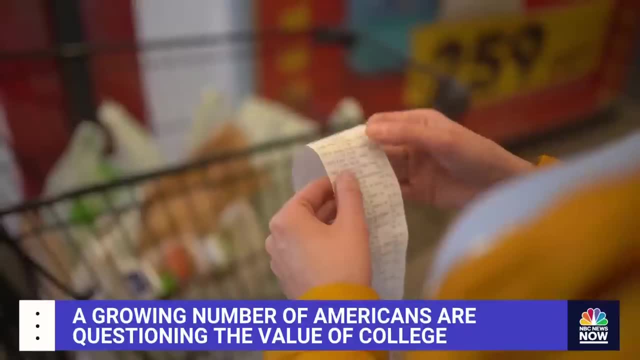 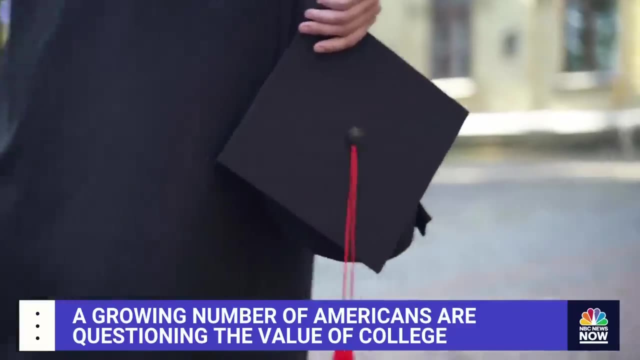 at colleges. We definitely know the struggle and feel that, but she's the one that pays for it. But now, in the middle of an ongoing pandemic and an economic downturn, more Americans are rethinking higher education's value. Two-thirds of Americans believe that you can find a well-paying job, a stable job. 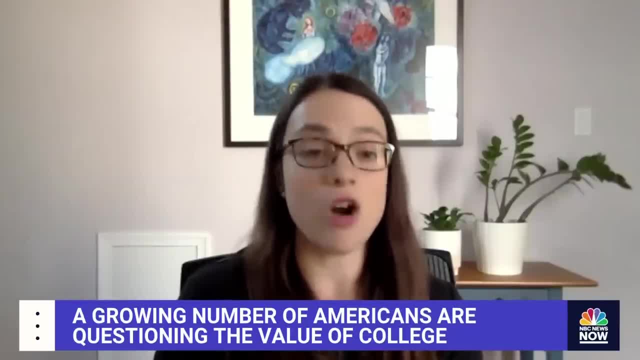 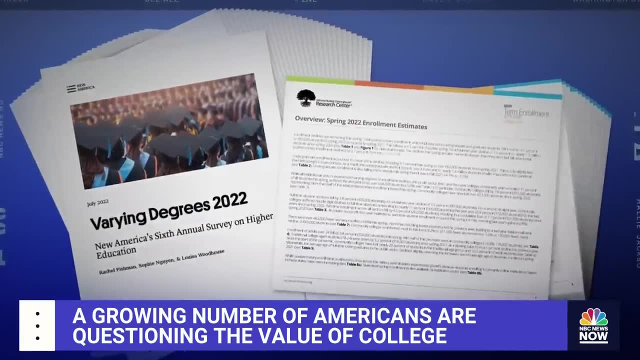 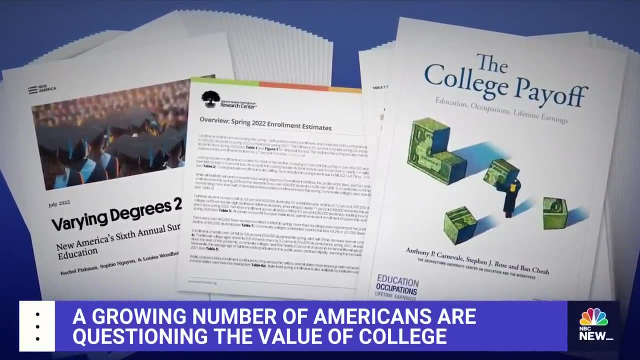 with only a high school degree or equivalent and no college education. That study by Think Tank New America adds to the growing trend of research showing that some Americans are either not going or not finishing college, in large part due to the increasing cost of getting a diploma. 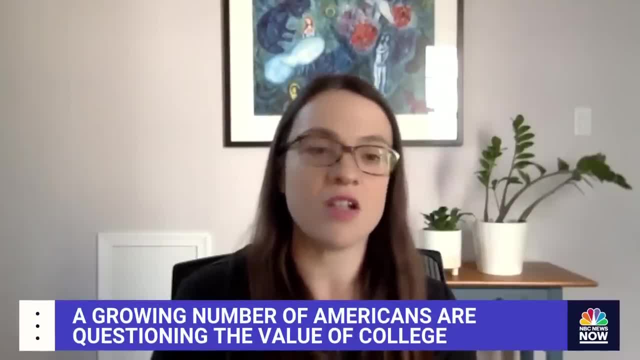 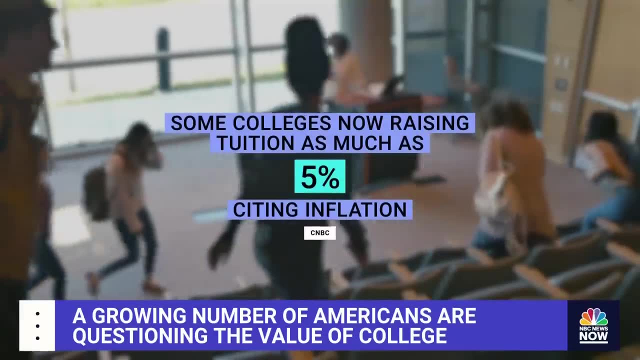 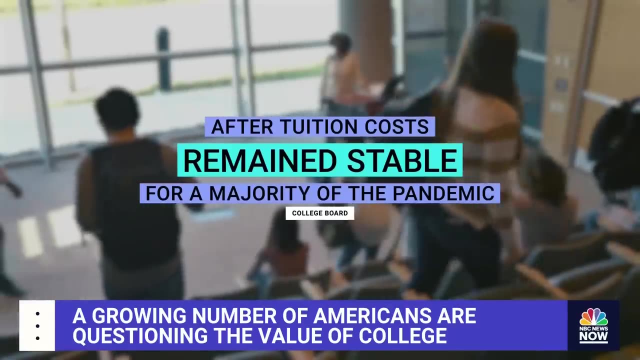 People are really trying to figure out what makes the most sense. Do I take time out of the workforce or can I work immediately with a good wage? Some colleges now raising tuition as much as 5%, citing inflation after tuition costs remain stable for a majority of the pandemic. 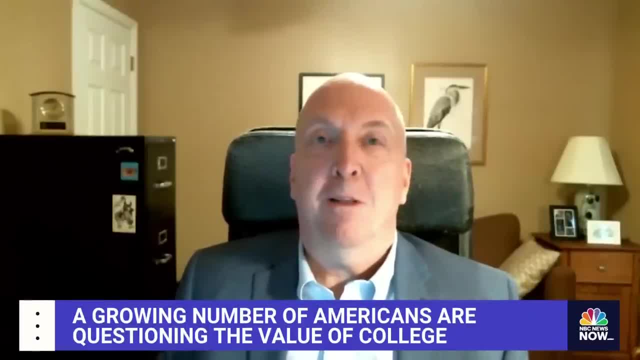 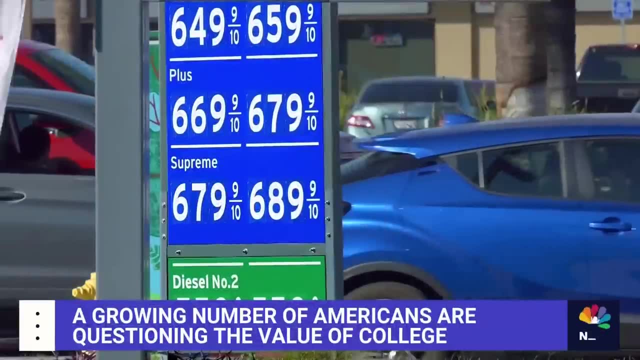 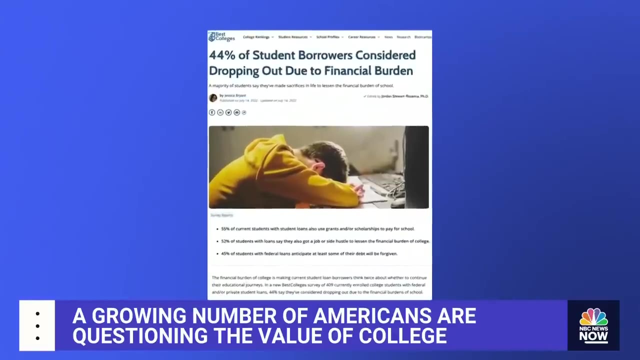 If you are thinking about enrolling in college or what the value proposition of college is and you're measuring the cost, you're measuring in terms of how many gallons of gas is it or how many eggs can I buy with what I would pay for this. A survey released this month by bestcollegescom finds 44% of. 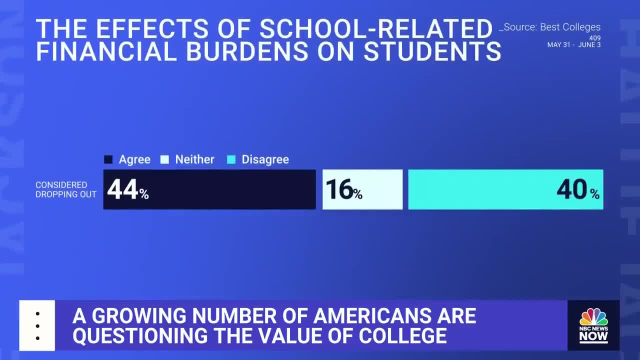 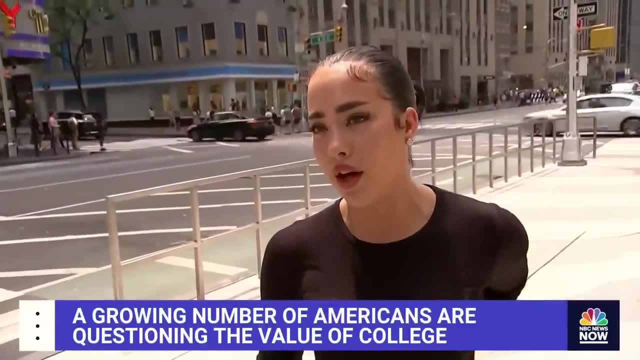 currently enrolled undergraduate students with federal or private loans have considered dropping out of school due to the financial burden. It's only worth it if you have an extremely high paying job as a result of that, like maybe law school, going into law after that, but a lot of other. 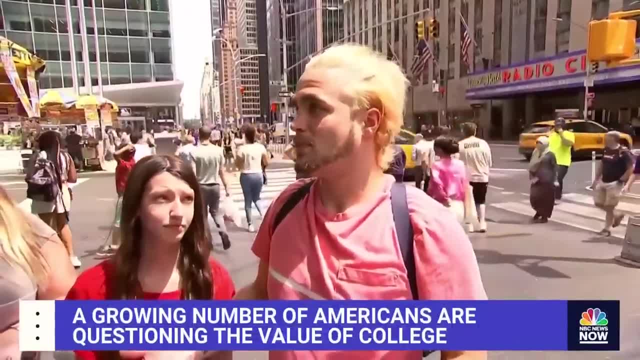 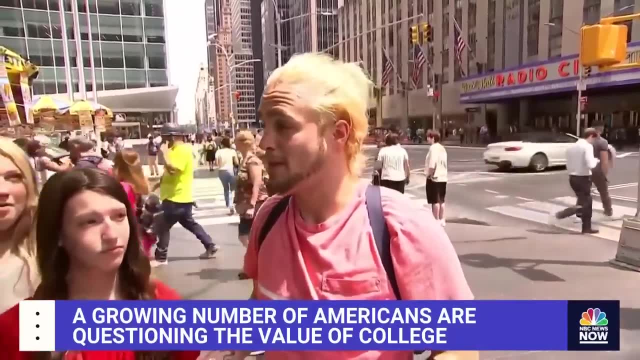 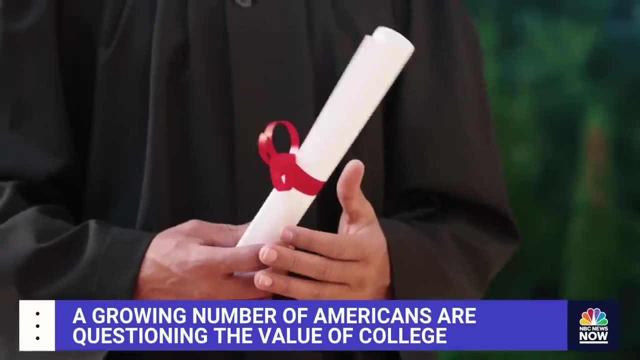 fields. it's not really worth it, in my opinion. I see my mom. she's still, 30 years later, still paying off college debt. so I mean I don't want to be in that position 30 years from now. The answer to: is college worth it? is unsurprisingly complex. Some research shows: 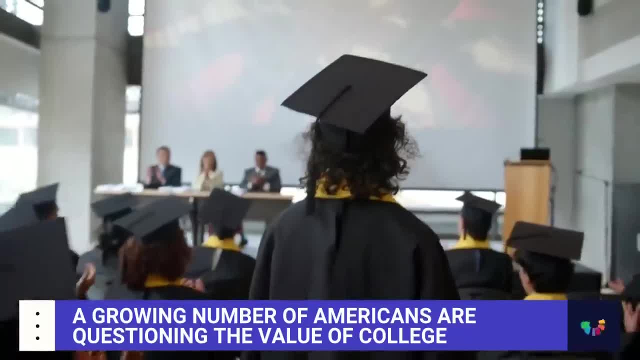 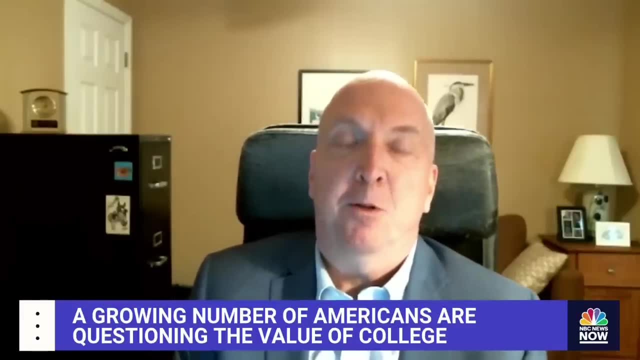 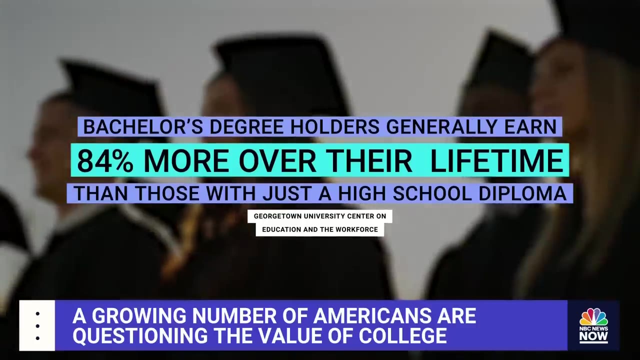 getting a diploma is worth it in the long run, especially for low-income students. That's sort of the sad paradox. College is most worth it for the people who can least afford it. A report Georgetown University shows, bachelor's degree holders generally earn a whopping 84% more over. 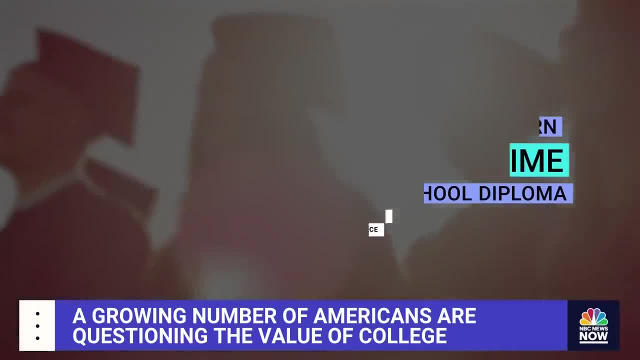 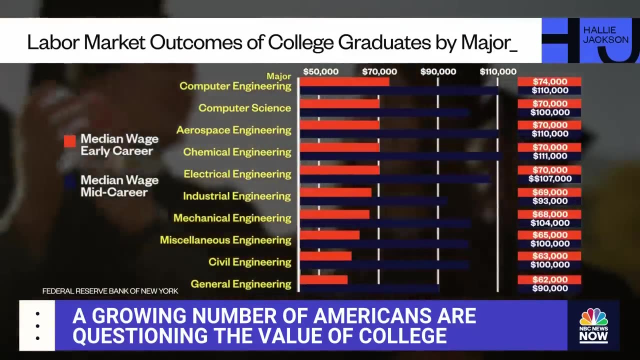 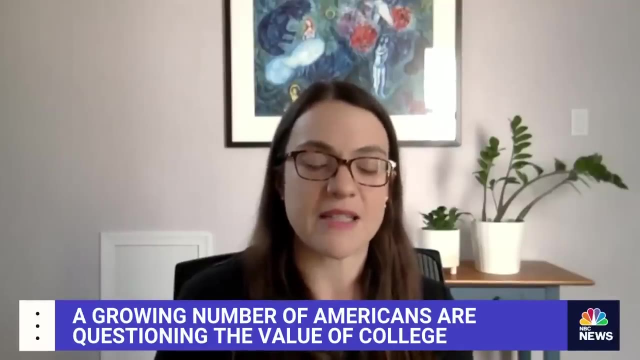 their lifetime than those with just a high school diploma. But nowadays the top 10 best paying majors are related to engineering or computer science, which represent just a fraction of the American population. Right now, the labor market's really tight. So if the labor market remains this, 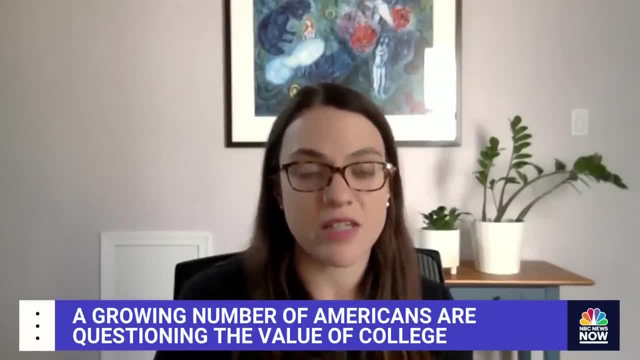 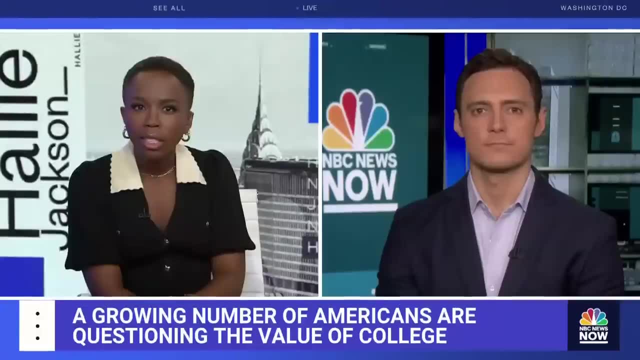 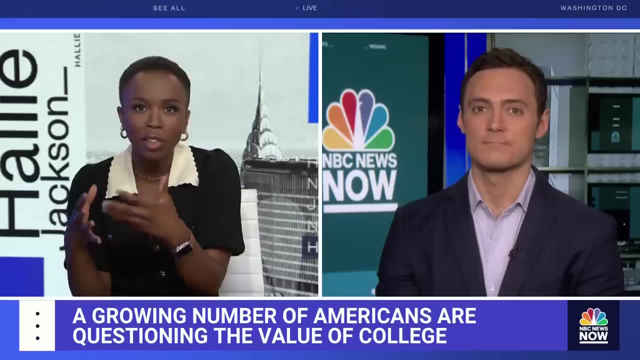 tight going into next year's survey, I think we'll continue to see numbers that change. Stephen, such interesting reporting. So many jobs, say today you know you need to have a master's degree or higher education college degree. So in your reporting I wonder, did you find that in? 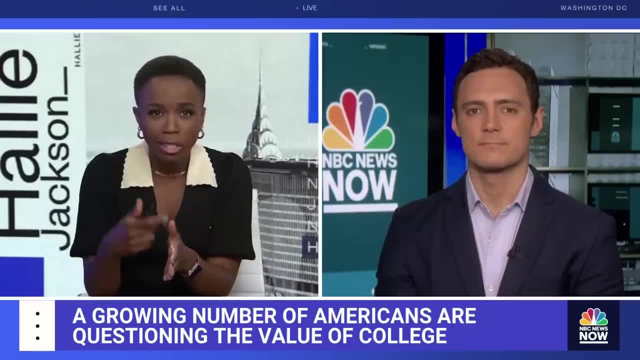 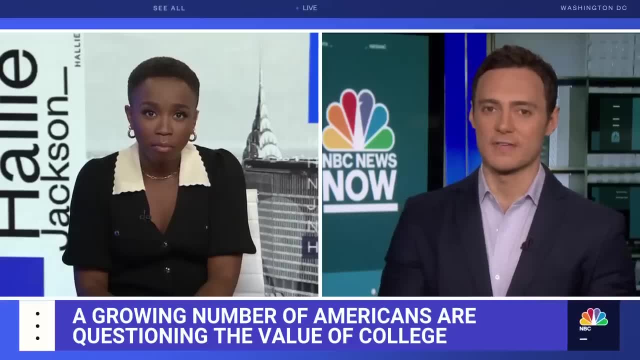 today's economy, foregoing higher education can actually result in stable, high-paying jobs. We heard a lot from people saying they don't want to go, but what are the results? Yeah, that's sort of the caveat to all of this. It can result in these high-paying jobs. 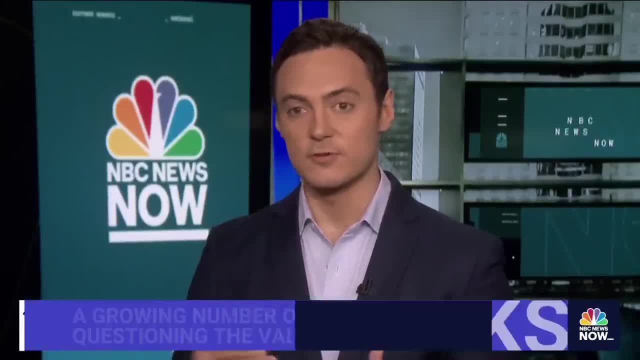 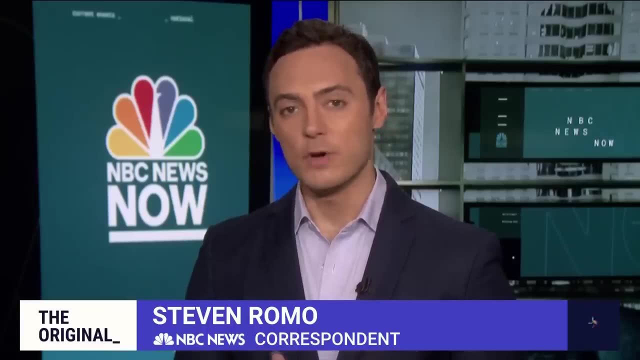 but you're at a much bigger risk in the economy right now if you don't have a college degree. That is still true. Some studies show that you can make up to a million dollars more over a lifetime with a college degree. Those things haven't changed, But people becoming more aware of 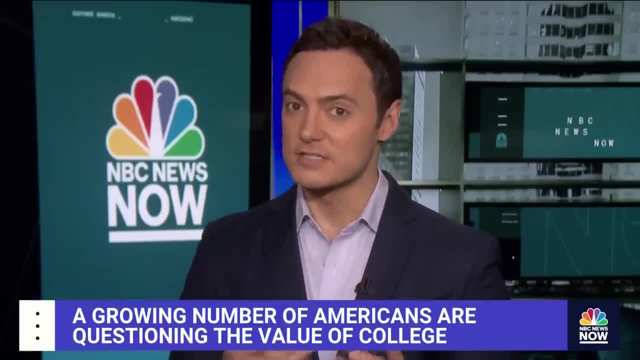 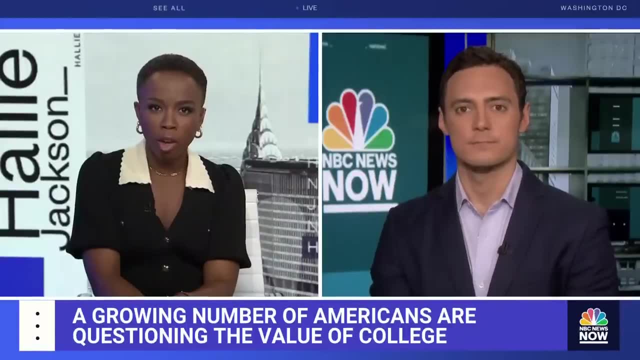 student debt and realizing that if they don't complete their degree, they're still going to be burdened with that debt is making them make these choices. And, Stephen, I mean it's impossible to talk about college without loans in the US. I don't know about you, I won't put you on the spot. 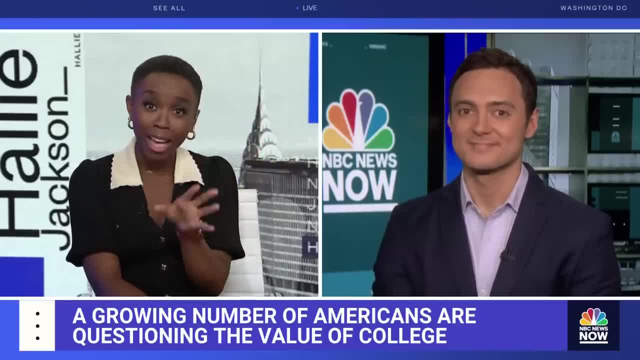 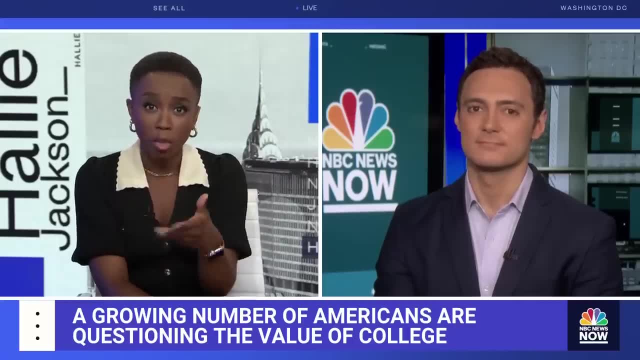 I know that I have, You know, a handful, And there's been lots of talk about student loan forgiveness being rolled out by the Biden administration. How might mass debt cancellation impact this trend that you reported on? Yeah, I wouldn't have been able to even step foot into a college without student. 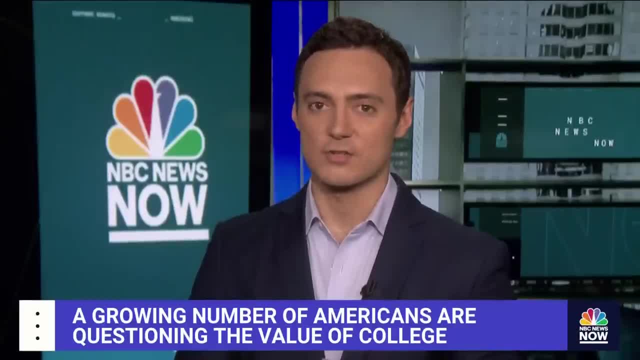 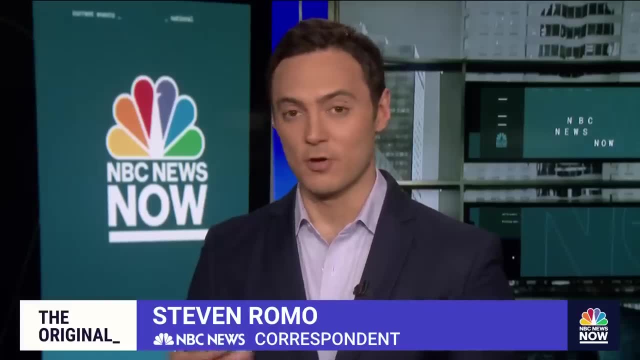 loans and student aids in clay. It is an interesting question. right now, Of course, it's still early on and student debt forgiveness hasn't actually taken place at a level that people are still asking the Biden administration for, So there's not a lot of information, There's not a lot of surveys being